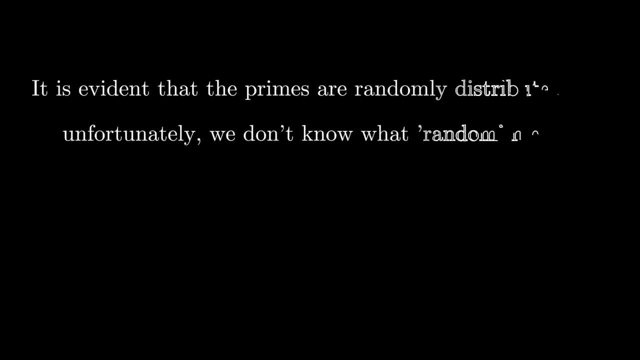 Here's an age-old question. Consider a sequence of prime numbers. So we have 2,, 3,, 5,, 7,, 11,, 13,, 17,, 19, and so on. Now, given a prime number, p, how would I predict the next prime number in the sequence? 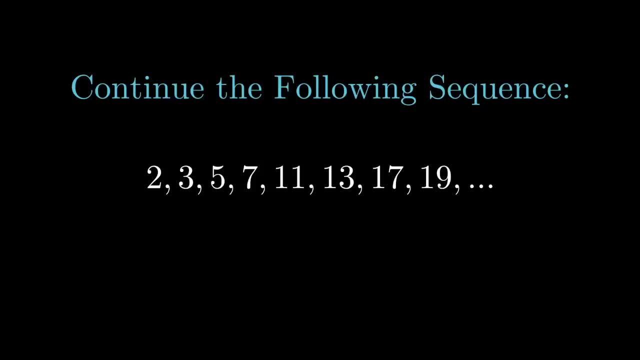 This question is actually incredibly difficult. It's the type of problem that, if you solve it, you would be among the math legends, like Euler, Newton or Riemann, Not to mention there's also a 1 million dollar prize for someone who can solve a related problem. 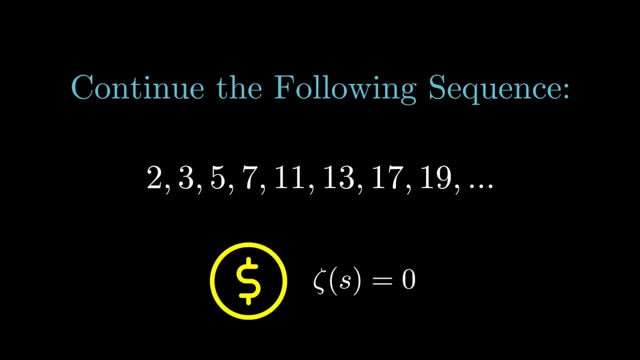 But just because this question is so difficult, it doesn't stop us from exploring the various things about the distribution of primes. Prime numbers are one of the simplest yet most complicated and confusing topics of math. Let's start from the basics. In middle school we learned that any number can be factored into prime numbers. For example, 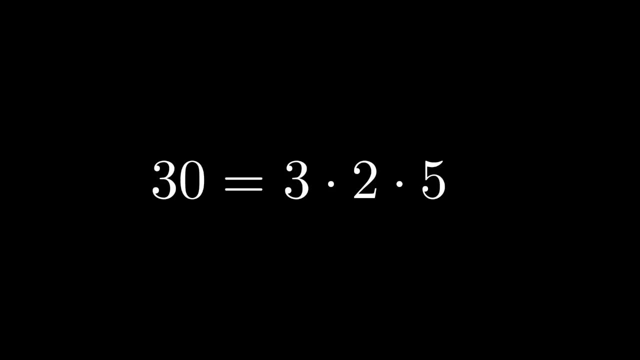 the number 30 can be written as 2 x 3 x 5.. So we have two types of numbers: primes and composite numbers. So Euclid's theorem is fairly straightforward. It just states that there are an infinite number of primes. So let's quickly go over a proof. This proof is actually pretty. 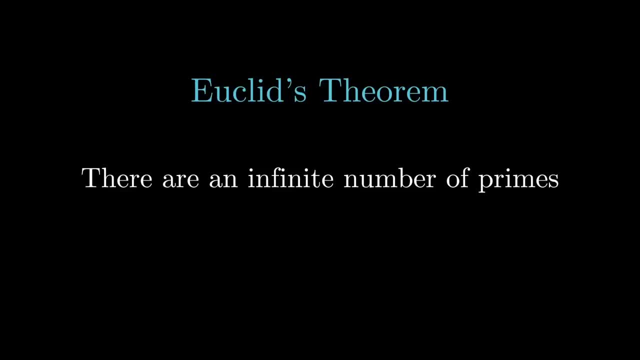 interesting. if you ask me, We're going to be using something called proof by contradiction. So first let's examine the proof of contradiction. We're going to use a proof of contradiction that the statement is false, that there are a finite number of primes. So let P 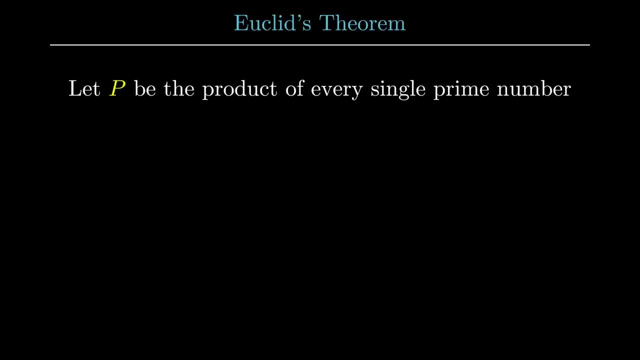 be the product of all of these prime numbers. So let's examine the number Q, which is equal to P plus 1.. So Q can be either prime or composite. So if it's prime, then we've already contradicted the fact that we found a new prime and 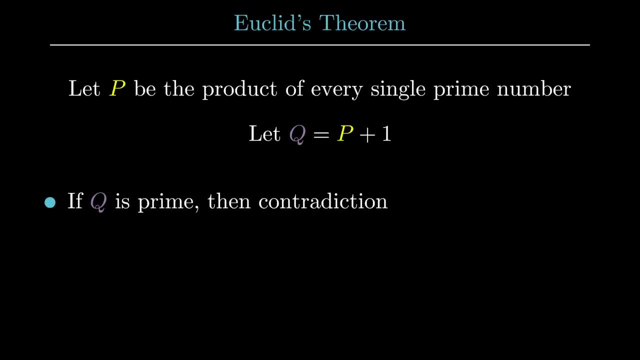 if Q isn't prime, then it has to be made up of prime factors. So let's look at one of those prime factors, P. and since P also divides capital P, it should divide P minus Q, which is equal to 1. and since no prime number divides 1, 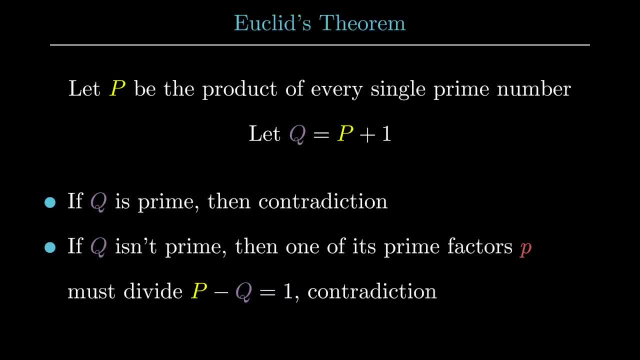 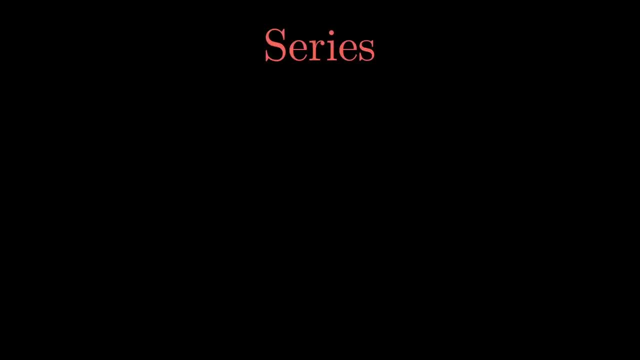 it's another contradiction, and so we've proved that they're an infinite number of primes. So before I talk about this, let's talk a bit about series. So series is just a sum of numbers. This is not to be confused with a sequence. An example of the series: 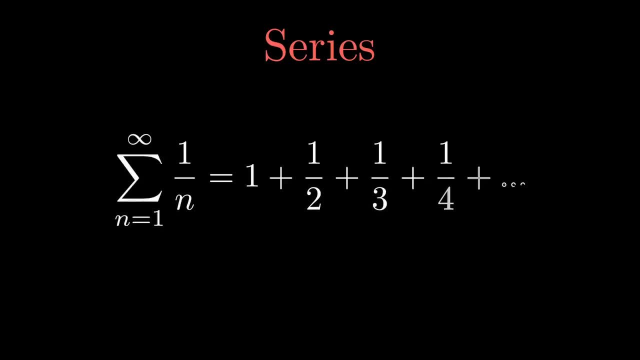 is the harmonic series, which looks like this: This series was shown to be divergent in the 14th century. What this means is that it does not approach a finite value. it just goes on to infinity, and I'll leave a link in the description. 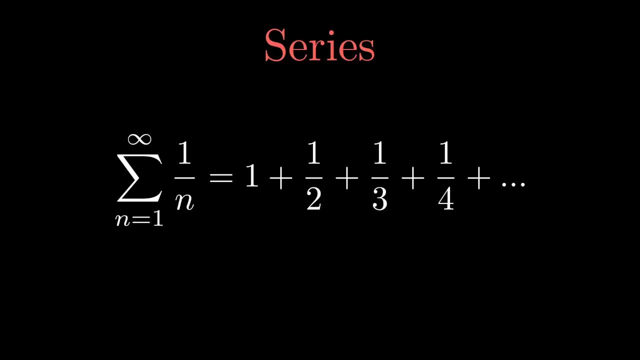 to how this is done if you're interested, but for now let's move on. A harmonic series is also known as a P series, which is a more general term, but the P value is equal to 1.. So the general formula for a P series is as follows. 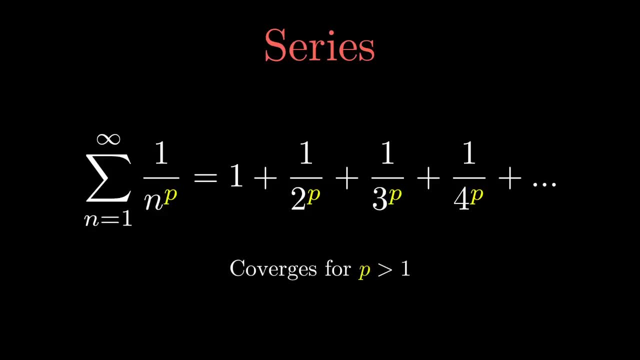 So P series always converge when the P value is greater than 1.. When I say converge, I mean that it approaches a finite value. So I'll leave a link to an article that shows why this is true, but it has to do with the integral test. So 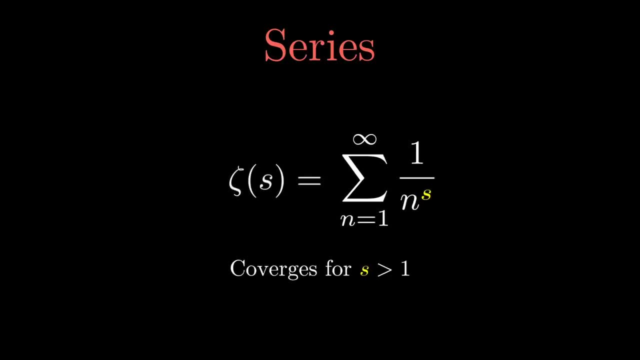 let's move on from that. So what we're gonna do is define something called a zeta function and this, essentially, the zeta function just gives a P series given a P value. But I hear you say: how does this have anything to do with the? 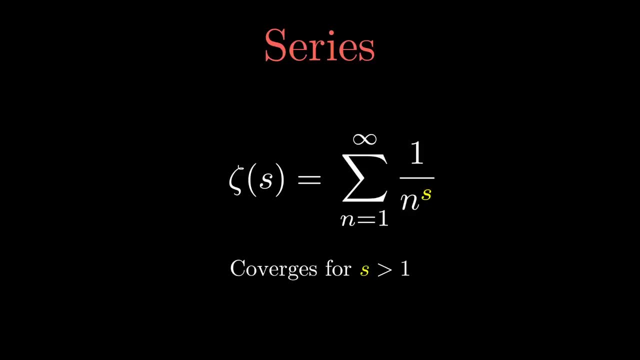 prime numbers. That's why we talk about the Euler product formula. but instead of just giving you the formula and talking about it, I want to discover it together. So let's just start off with the zeta function and its expansion. So we have this long formula, and then what I'm gonna do is I'm gonna multiply both. 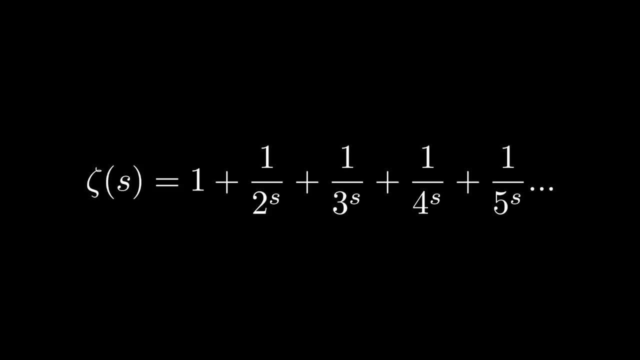 sides of the equation by the second term of the sequence. So in this case it's just 1 by 2 to the power of s. So you can see, on the right side we have every single multiple of 2 in the denominator. So 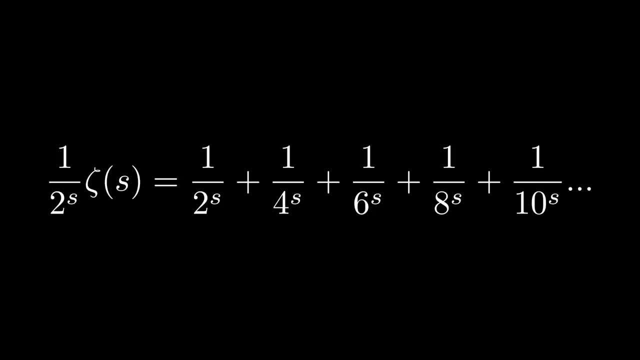 if we want to remove that from the original zeta function, we just do zeta of s minus 1 half to the power of s times zeta of s. So that's what we're gonna do and we have the remaining terms. Then we're gonna repeat the same process. 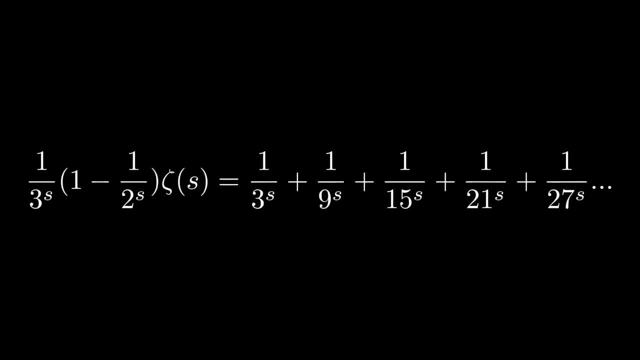 except for the second term of this new sequence. So we're gonna multiply both sides by the second term of the sequence now, which is 1 by 3 to the power of s. So if we do that, we have these terms and then we subtract them from the original. 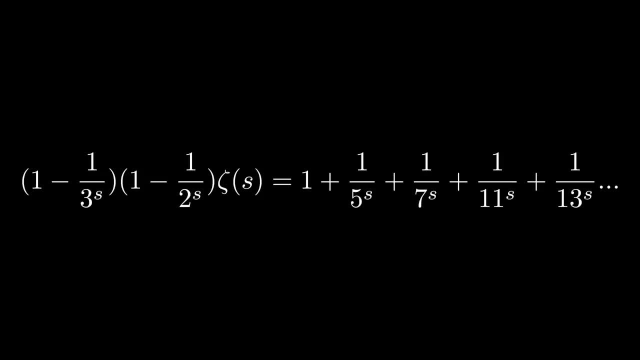 series, And then we do this again, and then, again, again. So if you notice that every time we do this we're subtracting multiples of each number, So the second term in our sequence is always gonna be prime. So if we continue this process to infinity, we get something like this. And if we move 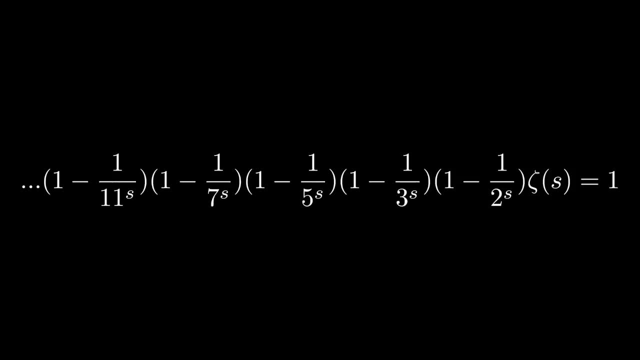 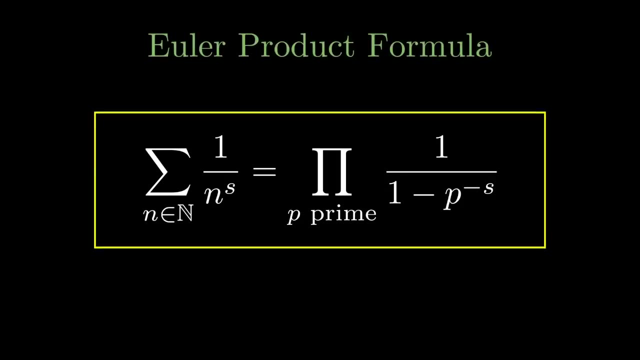 all the primes to the other side. writing this formally, we have sigma 1 over n to the s is equal to 1 over 1 minus p to the negative s for every single prime number. This is called the Euler product formula. It gives us the first relation. 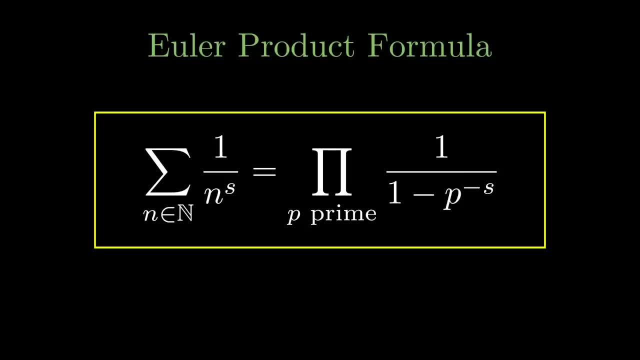 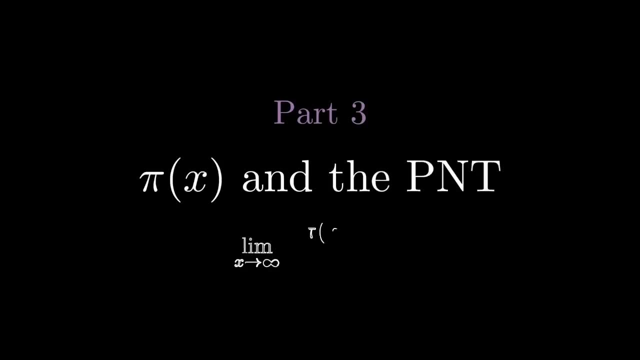 and prime numbers, And since this formula was discovered in 1737, modern study of prime numbers has always been based on the zeta function. The idea for the prime counting function is pretty simple. Let's give it a number x, Tell me the number of. 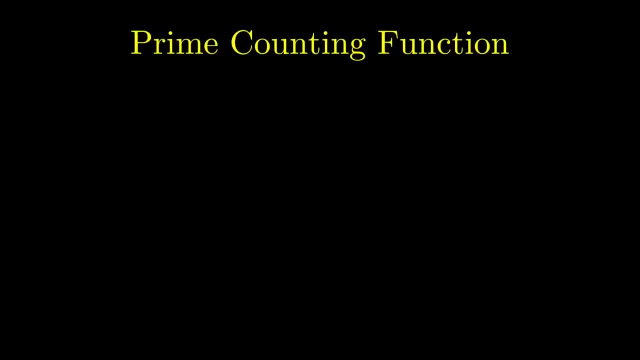 primes below that number. And this might be confusing, but we actually denote this function by the character pi. So a few examples are: pi of 5 is 3, pi of 10 is 4, pi of 20 is 8.. So the prime counting function is a step function means it's. 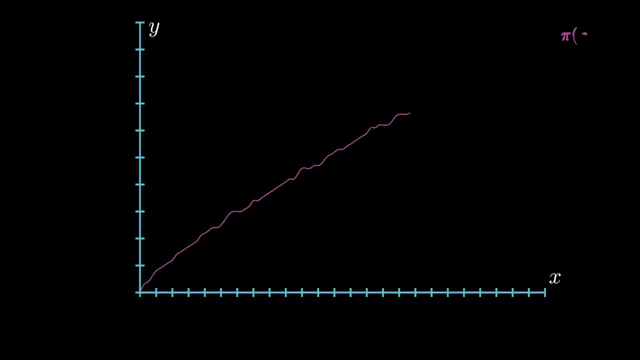 not continuous. So let's look at the graph of the prime counting function. And this function was introduced by Gauss in the 18th century. And another thing Gauss showed was that you could approximate the value of the prime counting function with the expression x divided by ln of x. This fact is called the prime number. 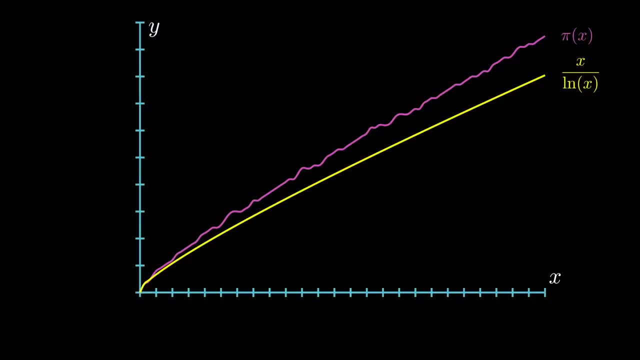 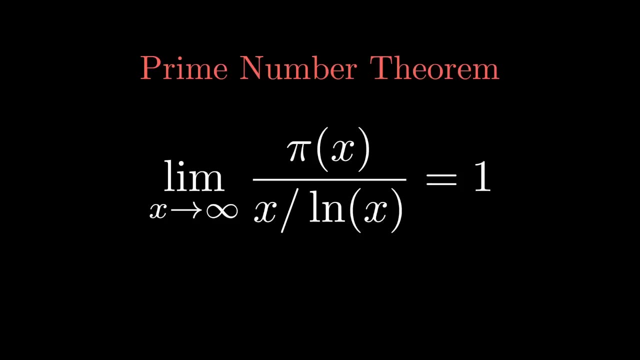 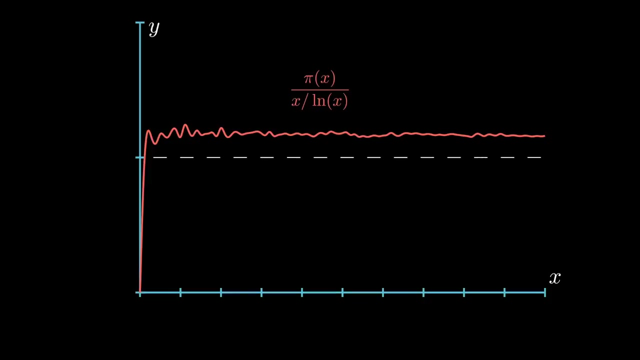 theorem More formally written, it states that the limit as x approaches infinity of pi of x divided by x by ln x is equal to 1.. So if we take a look at this graph- that's pi of x by x, by ln of x, you can see how it closely approaches 1. 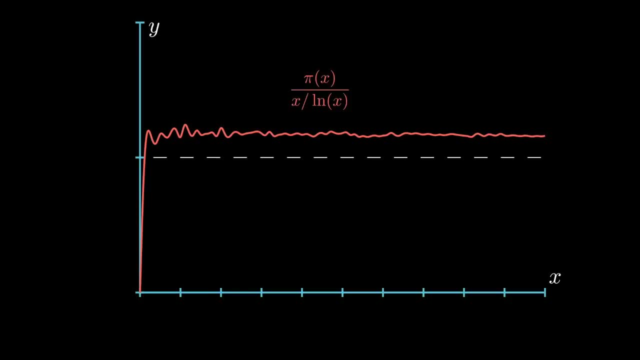 as x approaches infinity. So another result we can take from the prime number theorem is that the probability that a random chosen number is prime is roughly 1 by ln of x. In terms of the prime counting function. the prime number theorem tells us that each average step in 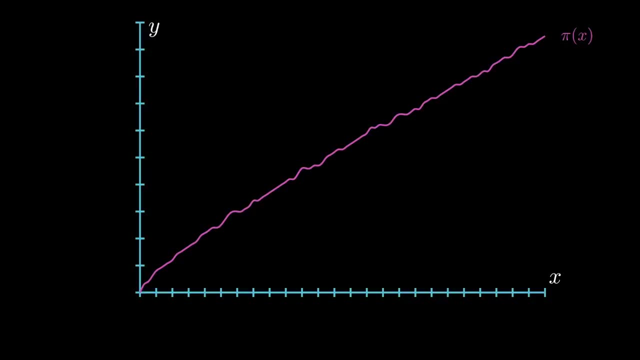 the prime counting function is around ln of x. However, there's actually a better function to approximate the prime counting function: What's the indefinite integral of 1 over ln of x? So my first instinct would just be to: oh, let's just plug it in in. 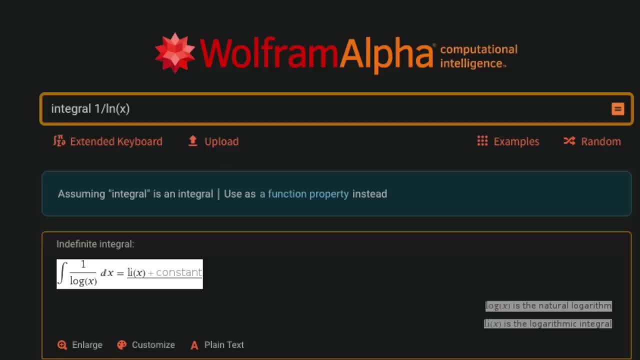 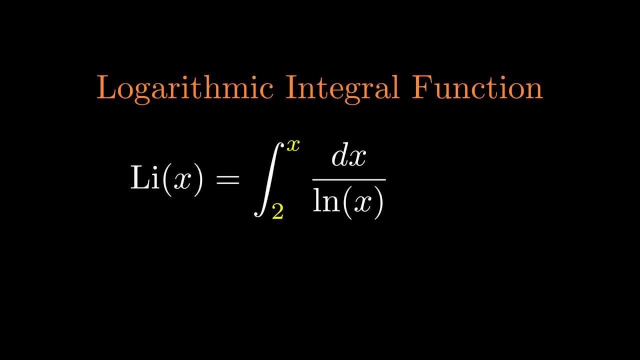 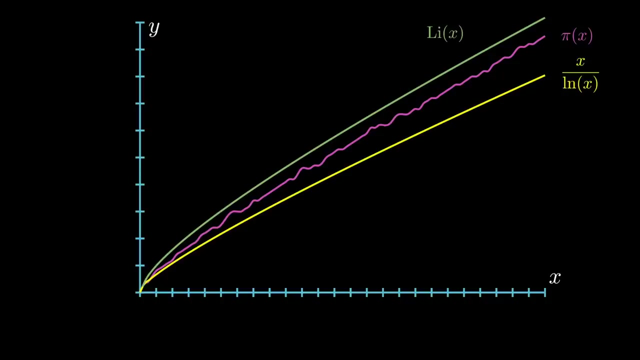 will from alpha. So I did that and we get li of x plus c. This li function is called the logarithmic integral. The indefinite integral of 1 over ln of t cannot actually be described algebraically, so we use this special function to describe it. It actually turns out that li of x is: 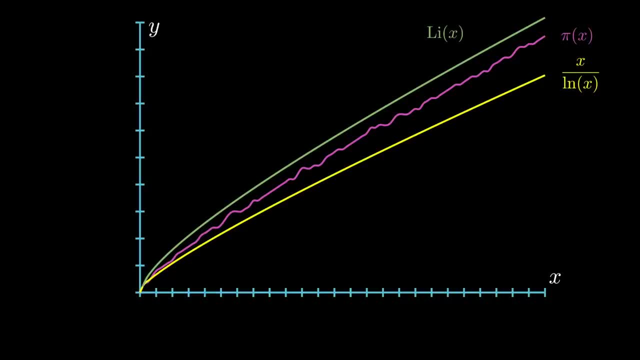 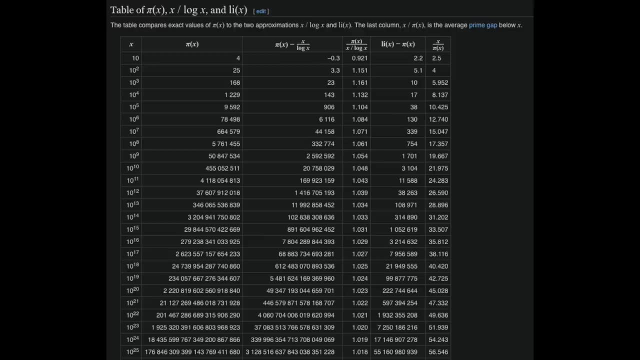 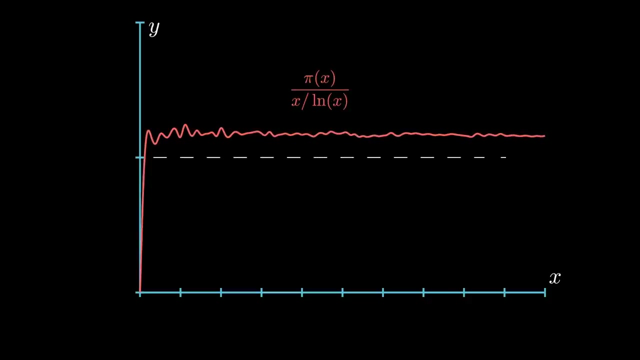 a better approximation for the prime counting function than x by ln of x. Here let's look at all three of them graphed. Wikipedia has a nice table that shows numerically why this is true. You can pause and take a look at this table, but for now I'm just going to skip it. Now let's go back to the prime. 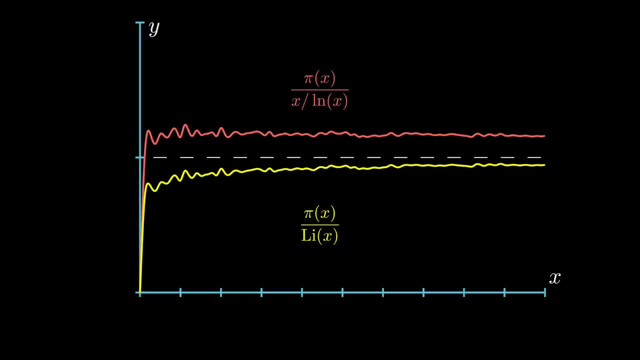 number theorem. Since li of x approximates pi of x, the limit as x approaches infinity of pi of x divided by li of x is equal to 1.. This way of approximating the prime counting function by the logarithmic integral function was discovered by Dirichlet after Gauss mailed him his prime number theorem. 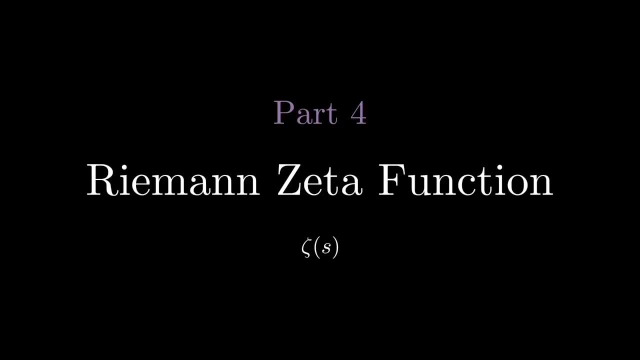 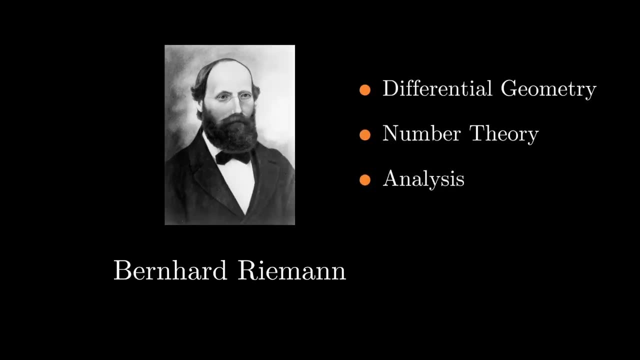 The Primer Number Theorem. Bernard Riemann was a German mathematician who studied fields like analysis, mathematics analysis, number theory and differential geometry. I'm sure you've heard his name before in your calculus class, for example, he came up with Riemann sums, So he was one. 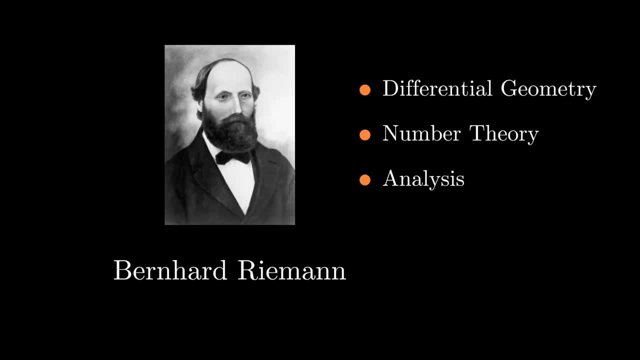 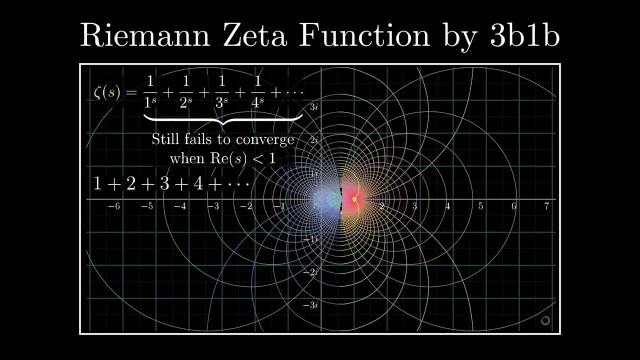 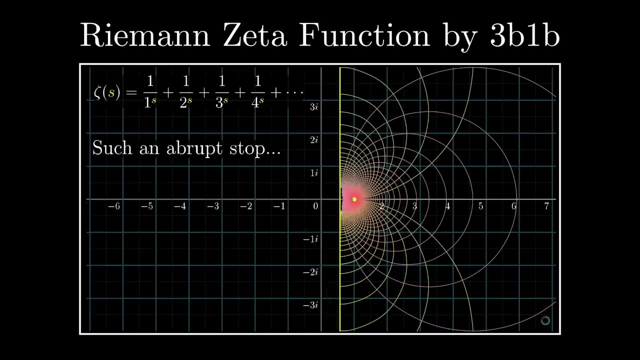 of the first to study what happens when you extend the domain of the zeta function from real numbers to complex numbers. So 3blue1bron has made a fantastic video on the Riemann zeta function and I think you should probably watch it. but let's quickly go over what the Riemann zeta function is. So the Riemann zeta function is essentially the zeta function that's used to calculate the value of a given number. The Riemann zeta function is essentially the zeta function that's used to calculate the value of a given number. The Riemann zeta function is essentially the zeta function that's used to calculate the value of a given number. The Riemann zeta function is basically the zeta function that's used to calculate the value of a given number. The Riemann zeta function is essentially the zeta function that's used to calculate the 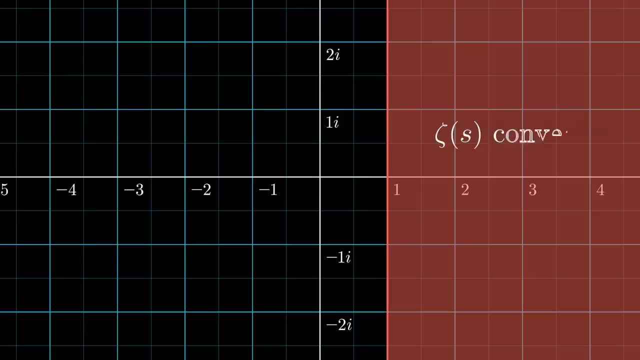 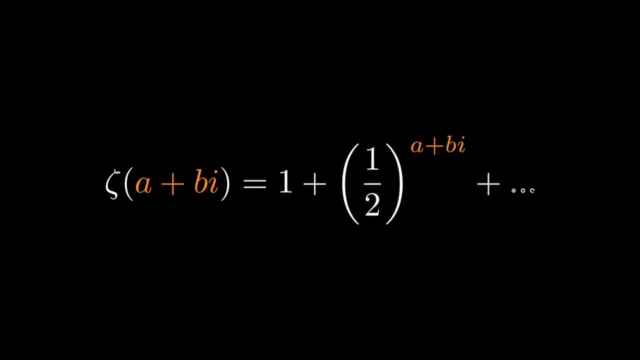 value of a given number. The data that's used to calculate a given addition can be researched to generate the sum. By using the demand hierarchy, we can plot the cál 경찰 to mantain the存 f satisfying in hexagon, And then what we see here is a Kraft. explore the Riemann方. 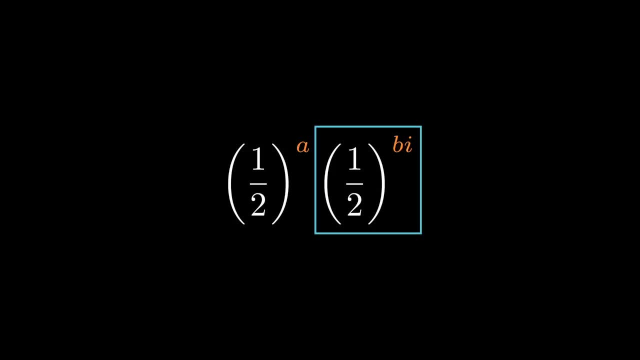 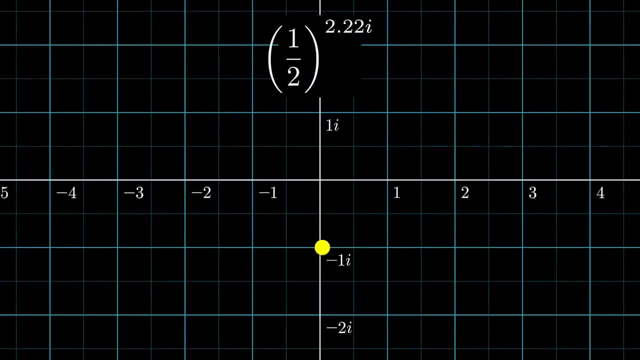 discoveries exponent, and what this turns out is that a complex exponent just accounts for some rotation along the unit circle with no change in the magnitude. I've left a link to a video by 3blue1brown again that explains this pretty well. but what this means for us is that the magnitude of each term in the Riemann 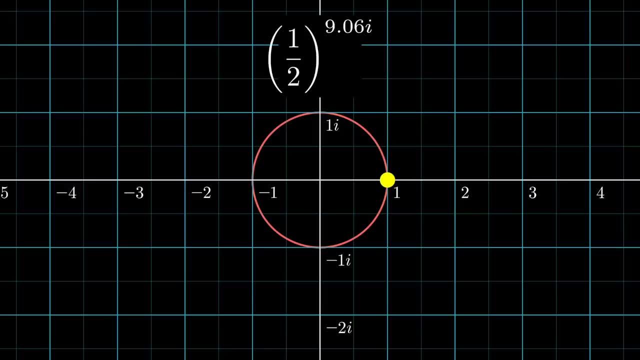 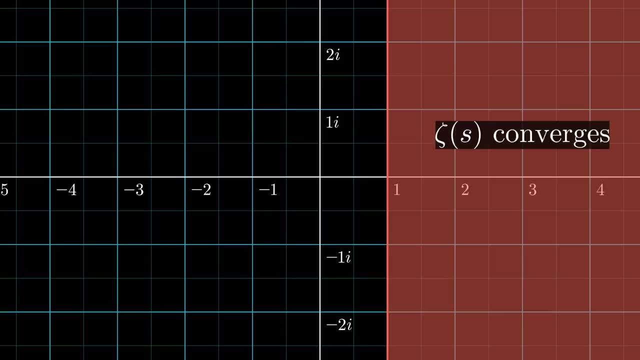 zeta function only depends on the real component, and so Riemann zeta function converges for Re which is greater than 1.. But what about the other side of the Riemann zeta function, where the real component is less than or equal to 1?? 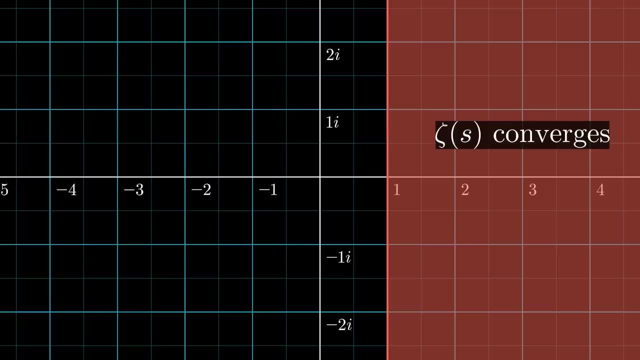 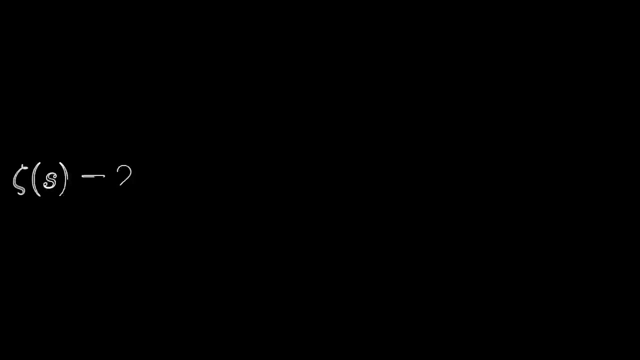 So Riemann used something called analytic continuation. Basically, he just extended the domain of the zeta function by quote-unquote, flipping it across across that line. So what Riemann studied was the zeros of the zeta function. So to examine this, let's look at the formula of this Riemann zeta function with: 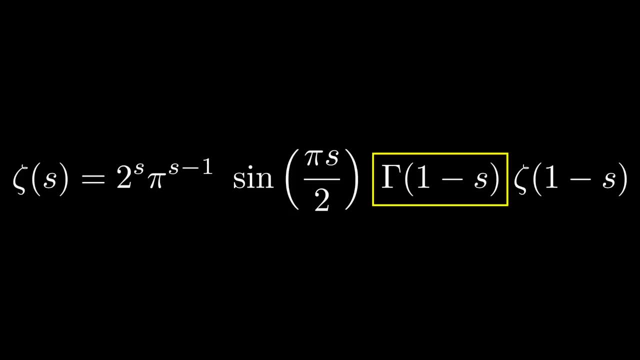 analytic continuation. So this term right here is the gamma function. See, the idea of the gamma function is that it's a function of the zeta function and the function is to provide a continuous function that goes through factorial points. Since I'm very lazy, I'm just gonna pull a clip from an old video of me. 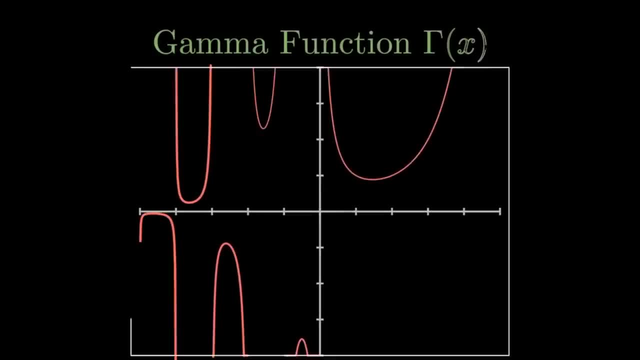 talking about the gamma function. The gamma function, which looks like this, is equal to n minus 1 factorial for all positive n. The gamma function is an extremely important function that appears all over math. It gives us a way to extend the familiar domain of factorials from positive integers to 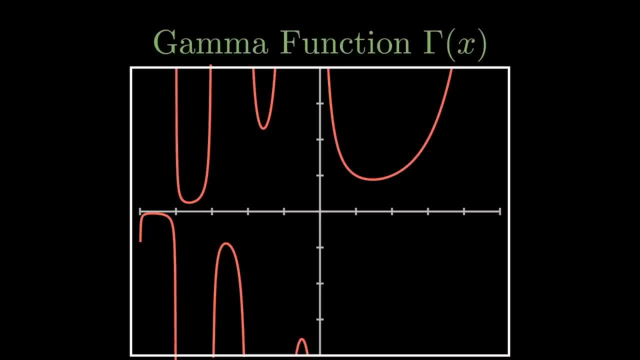 positive, real and even complex. real. Basically, the goal of the gamma function was to define a smooth curve that would go through factorial points. Here I've plotted three points which all satisfy: f of x is equal to n minus 1 factorial. So for x minus 1 the y coordinate is 1 minus 1 factorial, which. 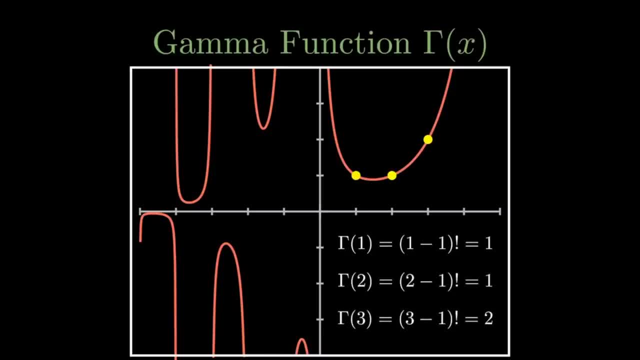 is 1.. Similarly, for x is equal to 2, the y coordinate is 2 minus 1 factorial, which is equal to 1. and finally, for x is equal to 3, the y coordinate is 3 minus 1 factorial, which is equal to 2.. 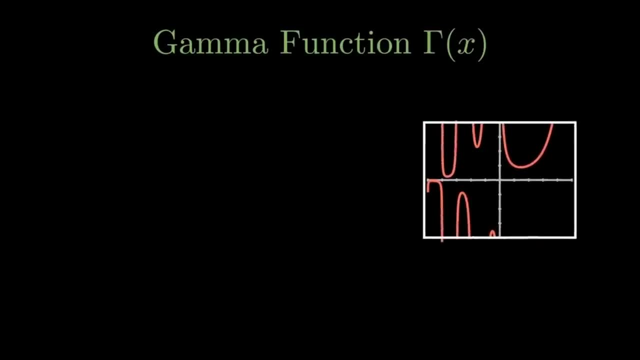 The gamma function is defined as follows: it's the integral, from 0 to infinity, of e to the negative t times t to the power of z minus 1.. Here's a challenge for you. try to see why this equals n minus 1 for positive integers. Hint, it has to do with 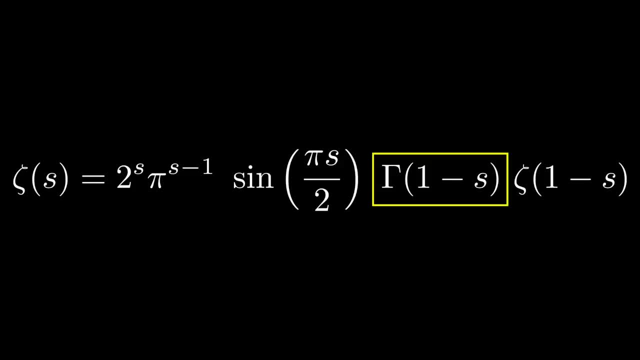 integration by parts. Thank you me from six months ago, by the way. if you haven't checked out that video, I highly recommend you do so. Going back to the Riemann Zeta function, let's take a look at the Riemann Zeta function. 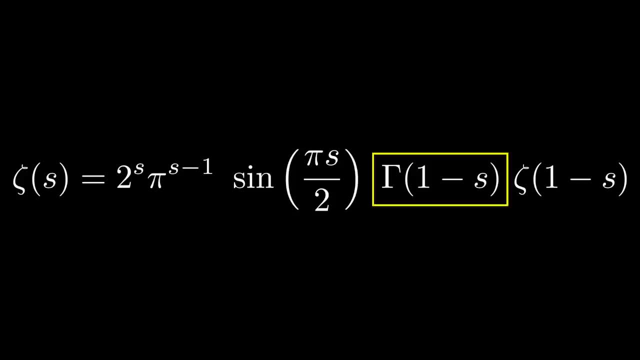 Look at the formula and see when it equals 0. So this sine term should equal 0 for all negative, even integers. These zeros are called trivial zeros. For positive, even integers, the gamma function forms something called a pole which cancels out the zero of the sine. 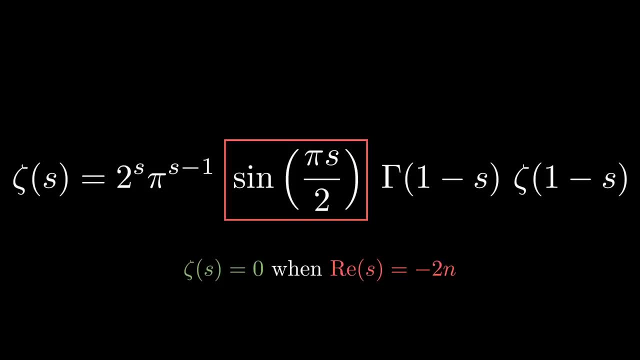 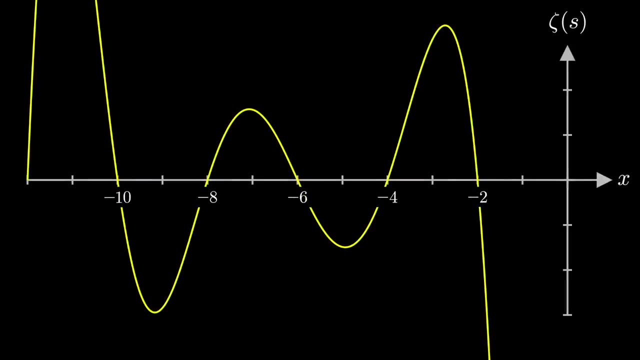 function. I'm not going to explain what this means here, but I've left a few links in the description to understand this. So a nice illustration of the trivial zeros of the Riemann Zeta function would be the graph If the real components of both the input and the output. look how zeta equals 0 at. 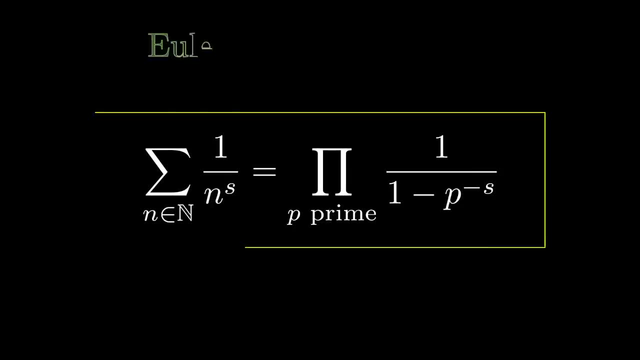 negative real numbers. So, going back to the Euler product formula, if the real component of the function is greater than 1, one of the products have to be equal to 0 for zeta to be equal to 0. And this is impossible because of Euclid's theorem which, if you remember, 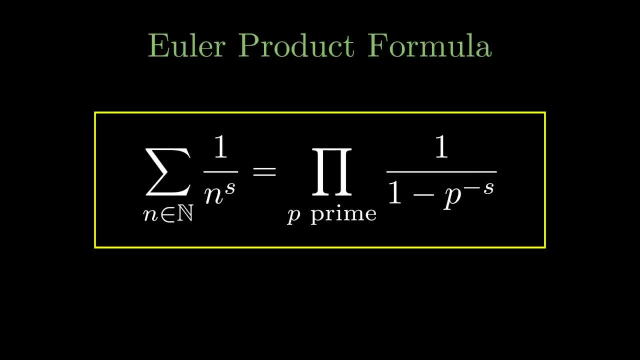 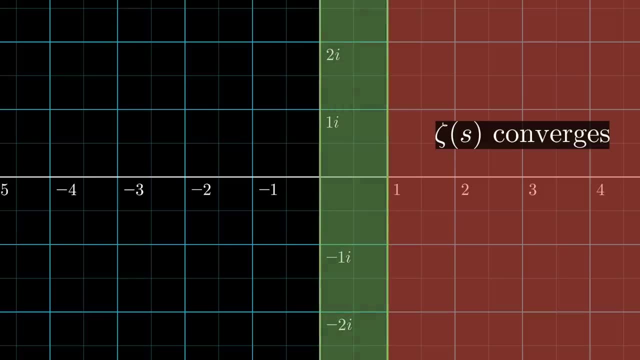 states that there are an infinite number of primes, so the right component cannot be equal to 0.. So the real components of the Riemann Zeta function have to have real component between 0 and 1.. So let's see if we can visualize them, The problem being that complex functions are pretty. 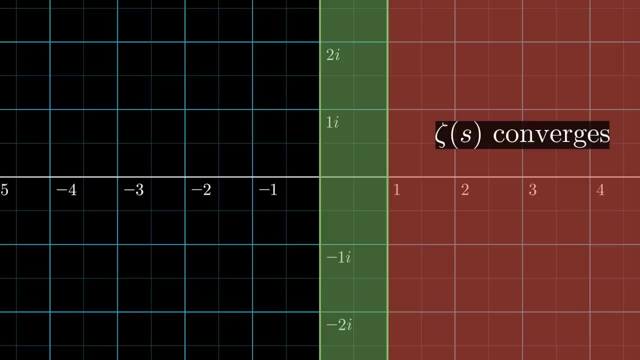 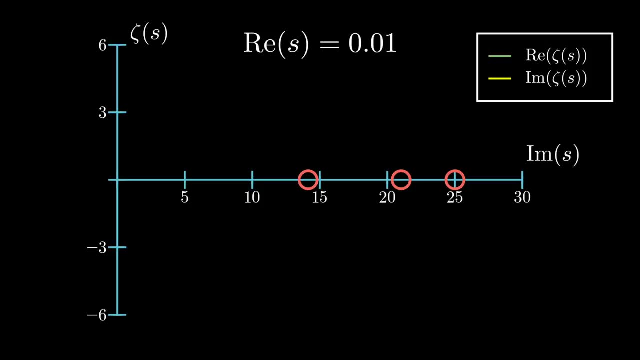 hard to visualize, but I'm going to try my best. So what we're going to do is we're going to fix the real component of our input and we'll have the x-axis be the imaginary component. Then we're going to have two graphs, one for 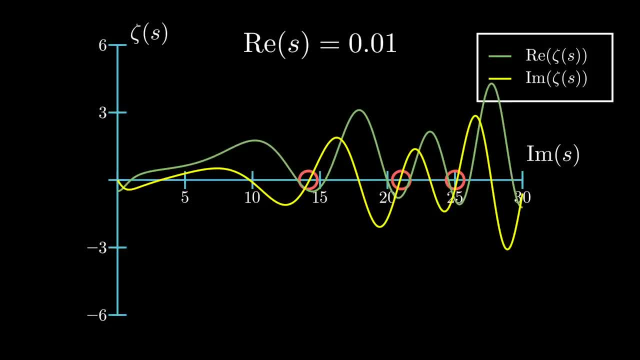 the real component and one for the imaginary component of our output. So, since we know that all the zeros we're looking for are between 0 and 1, let's vary the real component from 0 to 1.. I'm going to play the animation out. 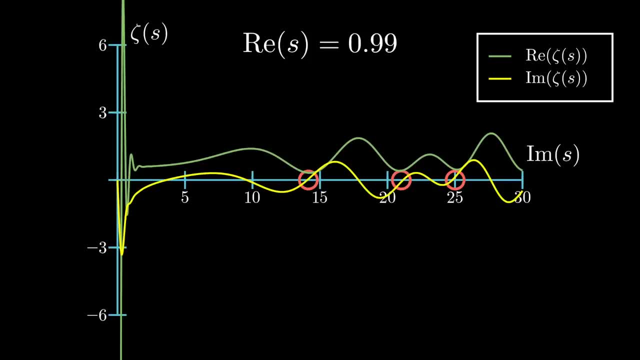 So now let's take a look at these red circles and focus on the red circles and play the animation once more. So, before we start, let's look at the imaginary component. Notice how it equals 0 at this point. Now let's play the animation. 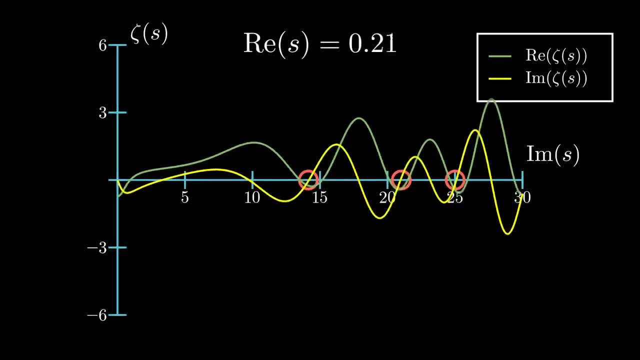 Let's play it once more. Stop. Notice that Re is equal to 0.5, the real component intersects with the imaginary component at 0.. Let's move a little bit more front to Re is equal to 0.6 and notice how there are no zeros. 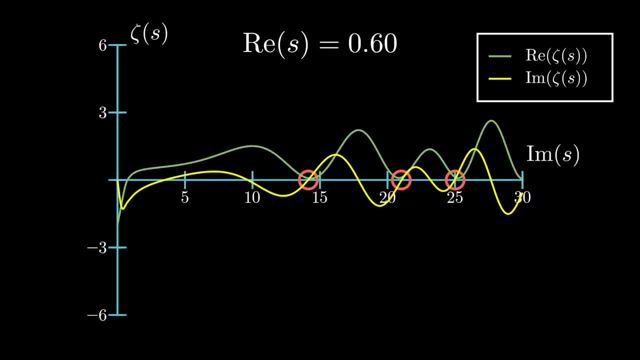 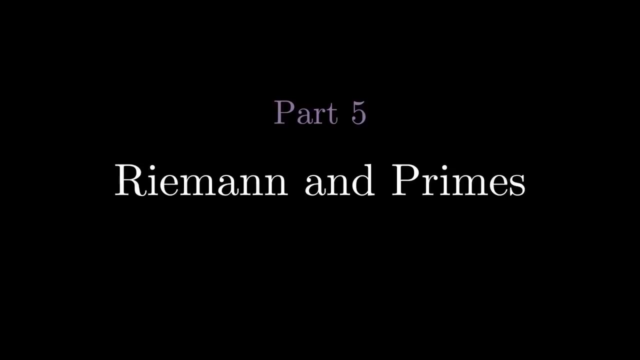 in the zeta function. So this is the famous Riemann Zeta function. It states that all the non-trivial zeros of the Riemann Zeta function have real component 0.5.. The clay math institute has offered a million dollars to anyone who can prove this fact. 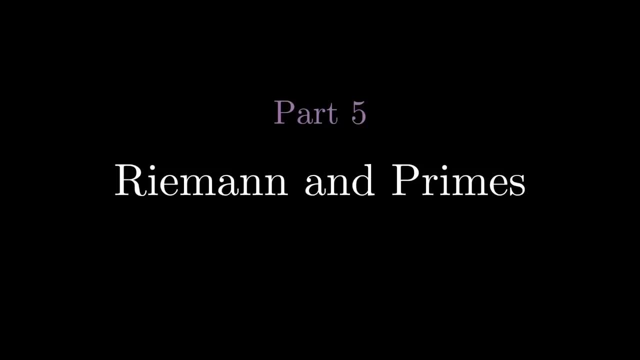 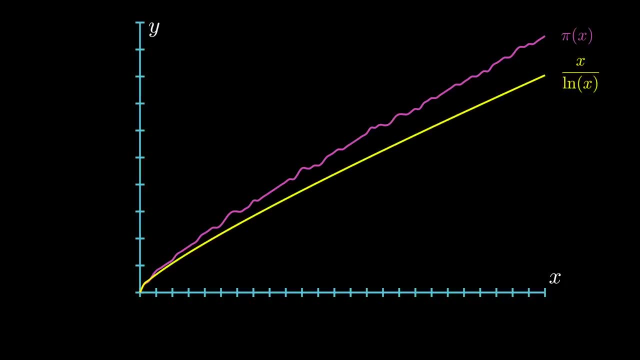 So I'm sure you're wondering how all of this has any connection to the prime numbers. So for this topic Let's go back to the prime number theorem. Remember how we could approximate the value of the prime counting function pi of x using the logarithmic integral function. 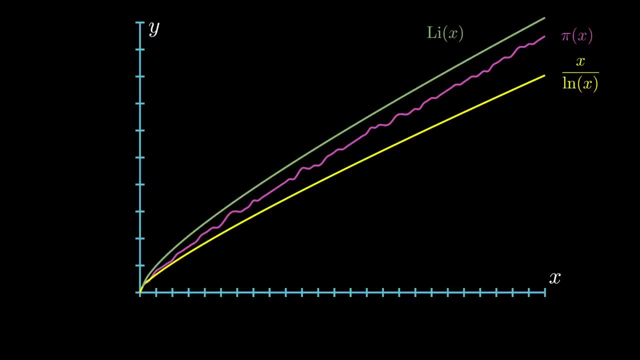 Well, the Riemann hypothesis helps us talk about the error by which the logarithmic integral function can approximate this function. If the Riemann hypothesis is true, this error is no more than some function of order. square root of x times ln of x. 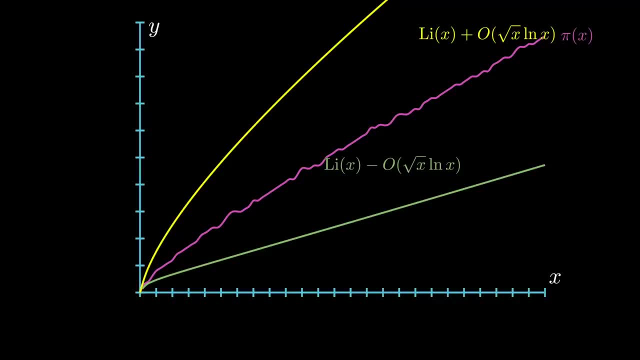 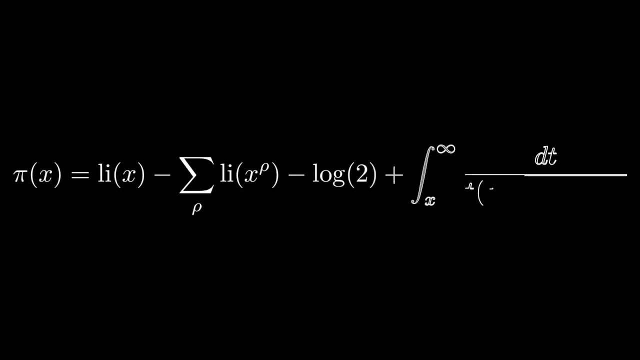 This goes both ways. We can prove that the error is a function of order: square root of x times ln of x A. more direct question is: how is the Riemann hypothesis? and primes is related. So this is where I talk about Riemann's explicit formula.